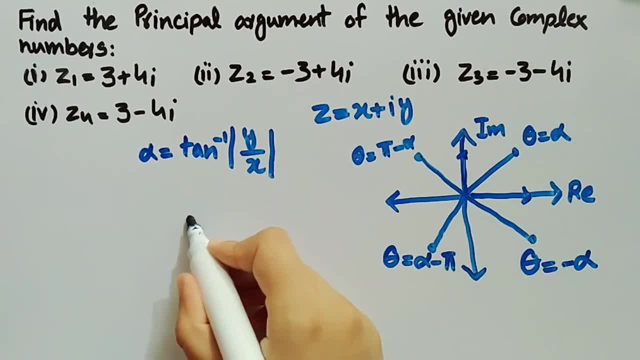 axis, then the principal argument, theta, which is represented by argument of z, where z is any complex number, will be equal to alpha. and if the complex number is on negative real axis or on negative imaginary axis, then the principal argument, theta, will be equal to minus times alpha. 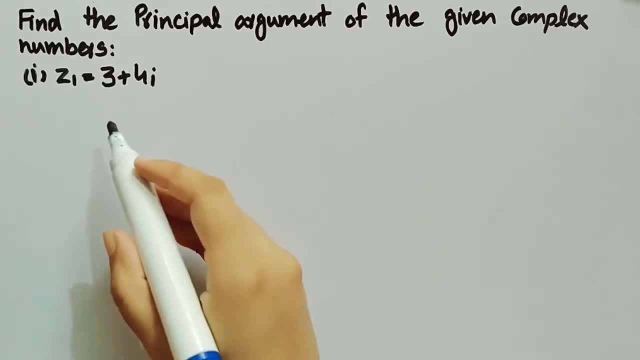 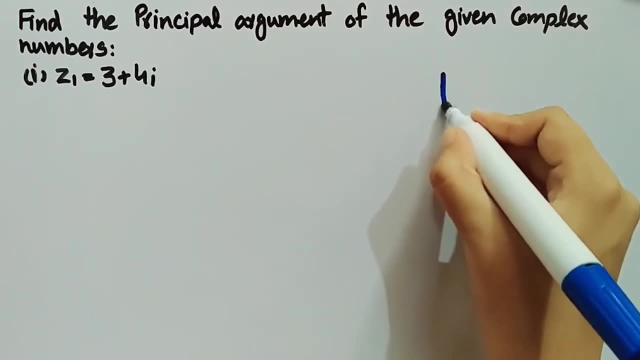 Now let's solve our first question, where z1 is equal to 3 plus 4 iota and we have to find the principal argument of z1.. Let's check that the complex number is in which quadrant? Let this be the real and this be the imaginary axis. The real part is 3 and the imaginary part. 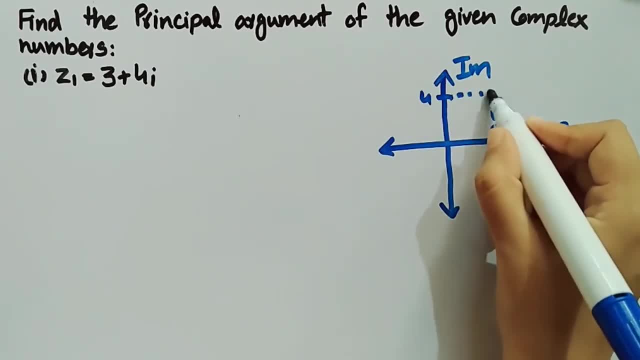 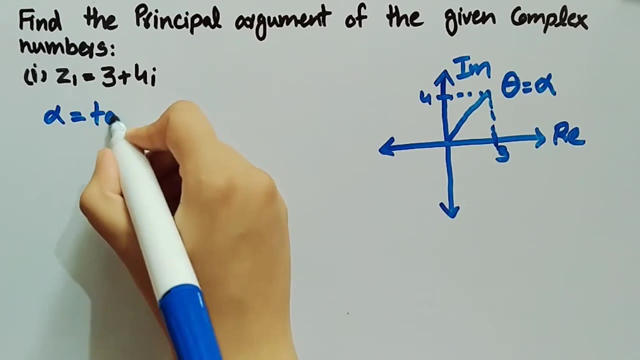 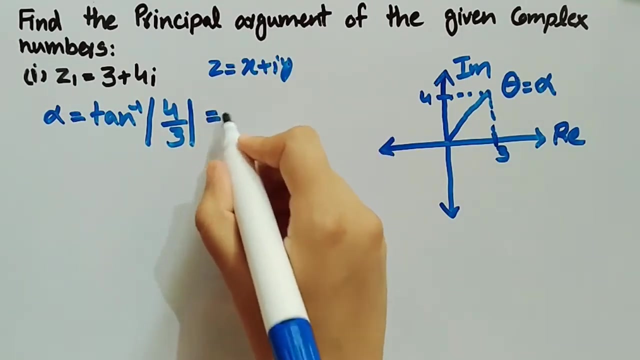 is 4.. So the complex number is in first quadrant. So the principal argument, theta, will be equal to alpha. Now we will calculate alpha, which is equal to tangent inverse 4 by 3.. 4 is y and 3 is x. for the complex number, zx plus iota y, which is equal to 53.13 degree. 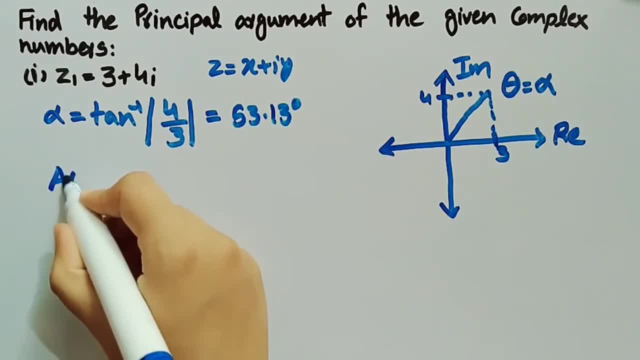 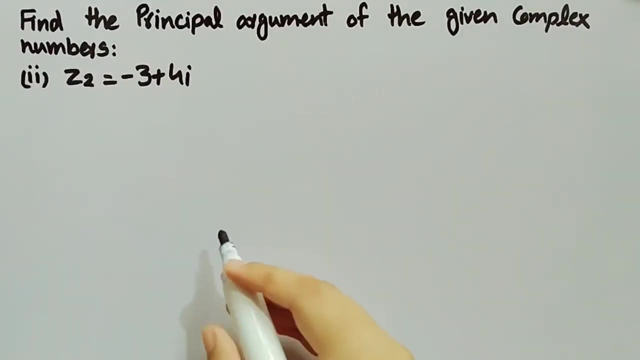 So in this case the principal argument of z1 is equal to alpha, so it is equal to 53.13 degree. Now consider the second complex number, z2, equal to minus 3 plus 4 iota. Now we will check that this number is in which quadrant. Let this be the complex plane and this be the real and this be the. 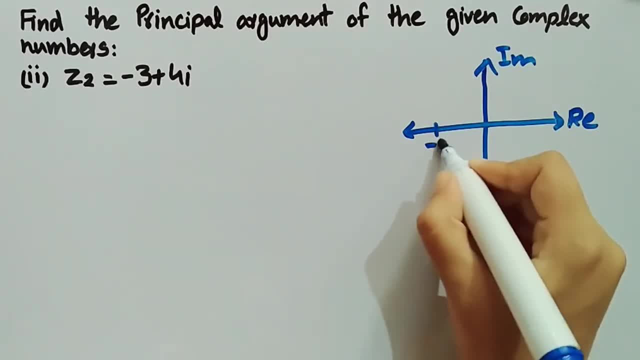 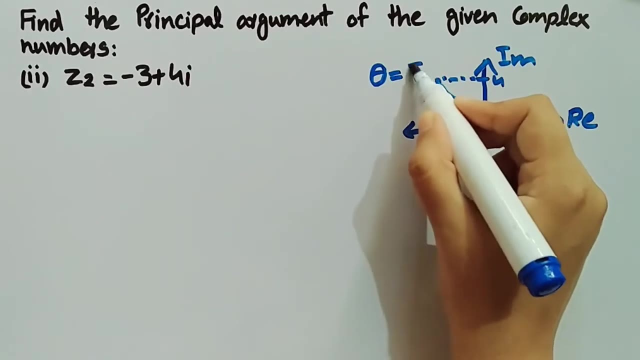 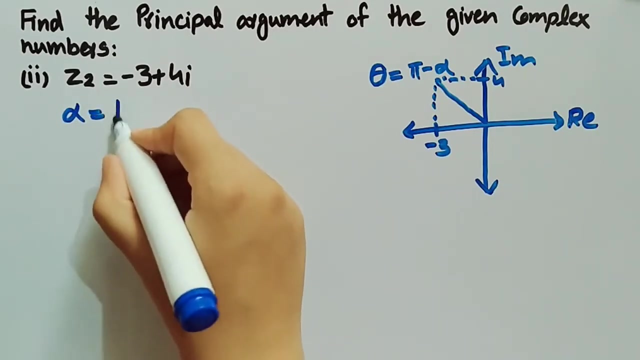 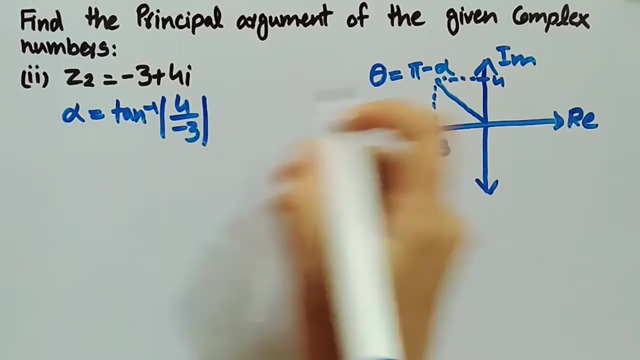 imaginary axis, The real part is minus 3 and the imaginary part is 4.. So the complex number is in which quadrant that this приعة is equal to h. So the principal argument of z1 is: Now we will find the value of principal argument of z2, which is equal to theta, which is equal 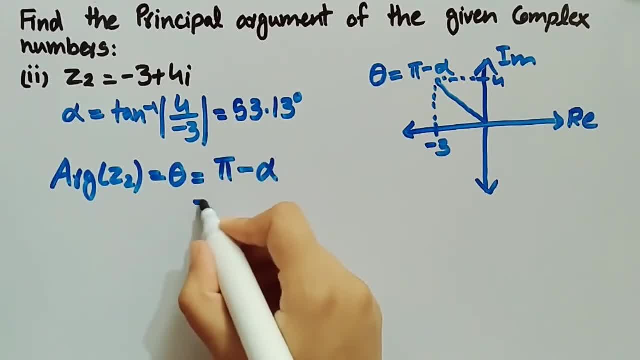 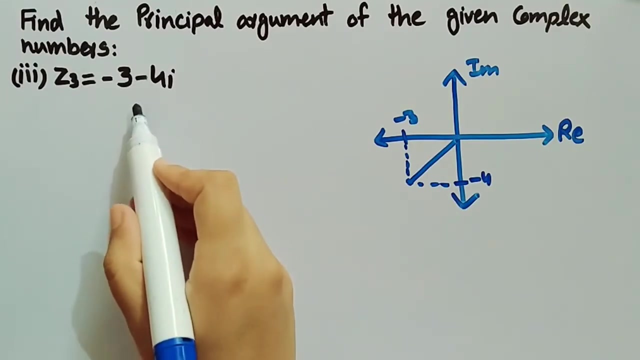 to pi minus alpha pi is equal to 180 degree, so we will substitute its value: 180 minus 53.13 degree is equal to 126.87 degrees. so this is the principal argument of the complex number z2.. Now consider the third complex number, z3, which is equal to minus 3 minus 4 iota minus 3 is 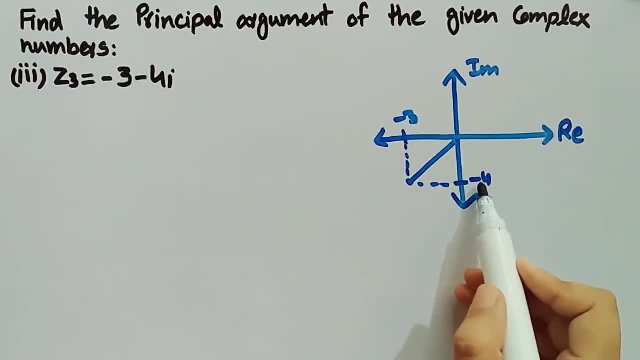 the real part of the complex number and minus 4 is the imaginary part of the complex number. So the complex number is in third quadrant. so the value of principal argument theta will be equal to alpha minus pi. so now let's calculate alpha, which is equal to tangent inverse minus. 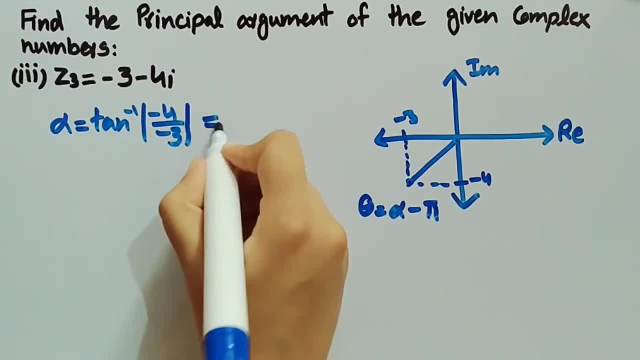 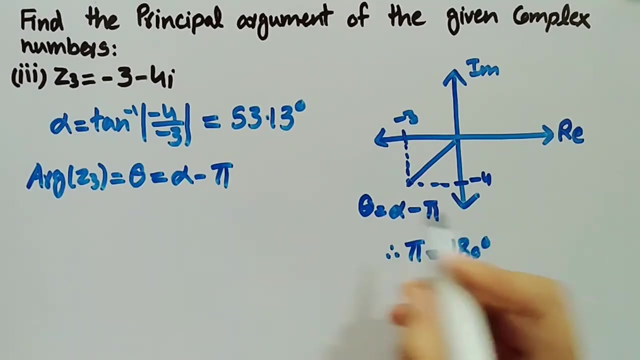 4 by minus 3, which is equal to 53.13 degree. Now we will calculate the principal argument of z3, equal to theta, which is equal to alpha minus pi. since pi is equal to 180 degree, Alpha is equal to 53.13 degrees minus 180 degree, which is equal to minus 126.87 degrees.